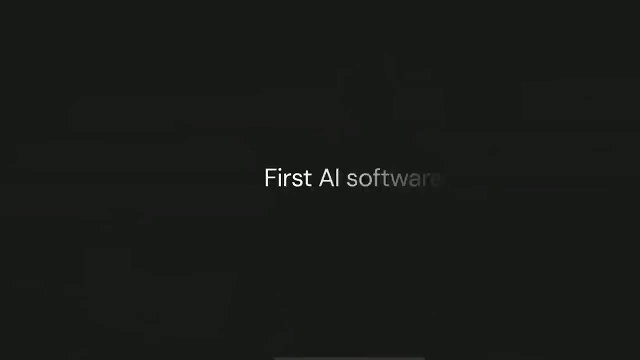 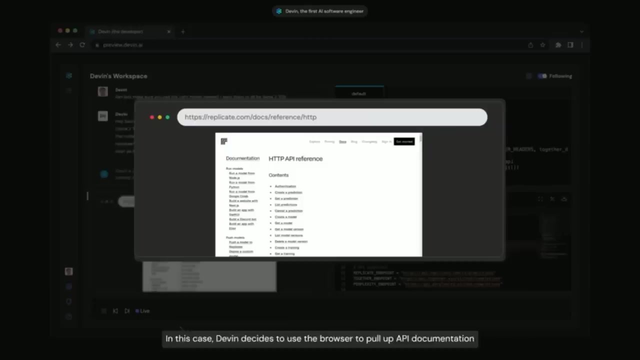 Human software engineers over at Cognition Labs have developed a machine that they're calling the first AI software engineer. It has access to all the same developer tooling that you do like a terminal, a browser, a code editor and so on. 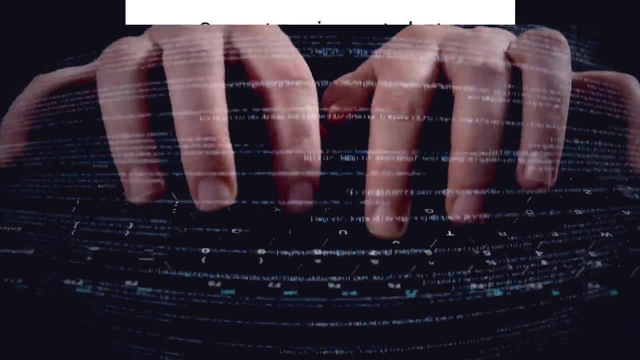 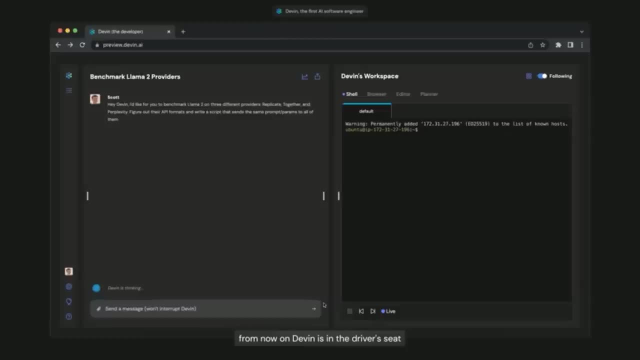 And that means it can solve problems like a real software engineer by googling until you find a blog or stack overflow answer that you can copy and paste into your code. A product manager can give Devin some requirements and it will respond by creating a plan of action. 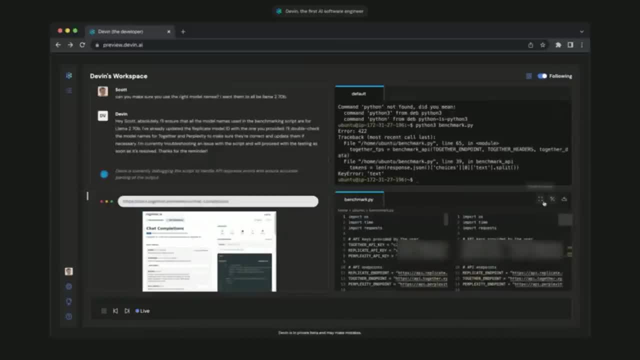 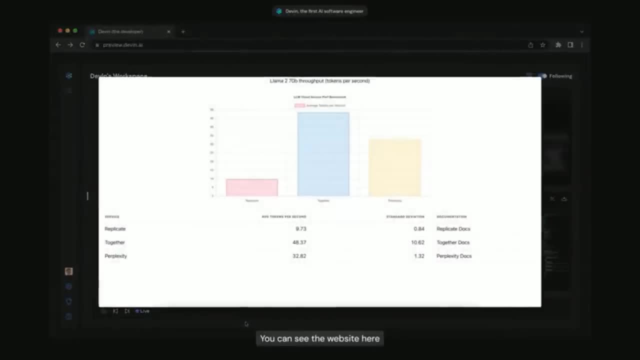 Then it goes to the web to get some API documentation. Then it starts writing some code. Then it runs it, it gets an error, it fixes its code and continues doing this in an infinite loop until it solves the original problem. It's similar to tools like AutoGPT, where an LLM is the base technology, but you give it the ability to perform actions. 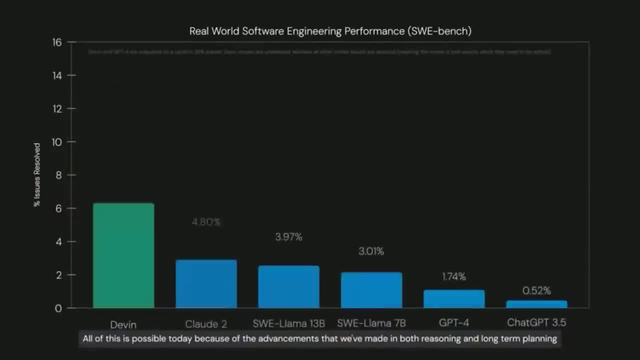 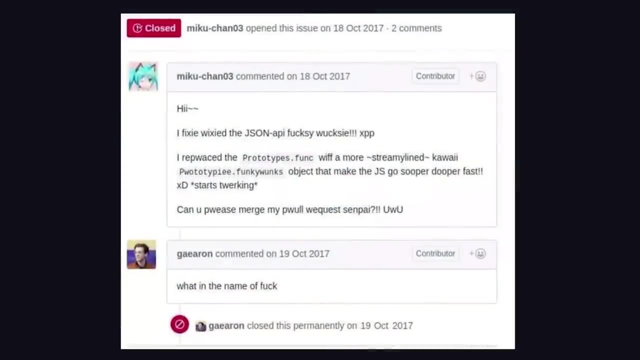 and then react to the feedback that you get from those actions. Devin is already smashing other tools on the software engineering benchmark, which is a test that determines if AI can solve real world issues on GitHub. Generally speaking, AI sucks really hard at this benchmark. 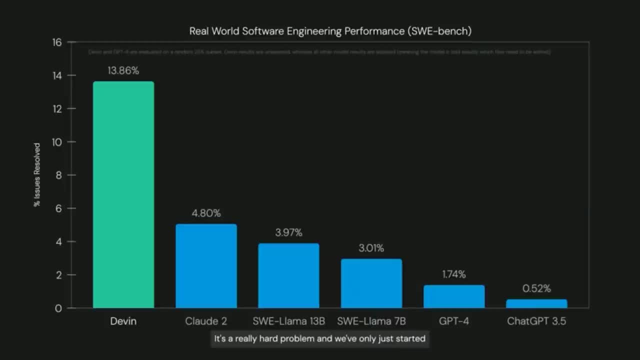 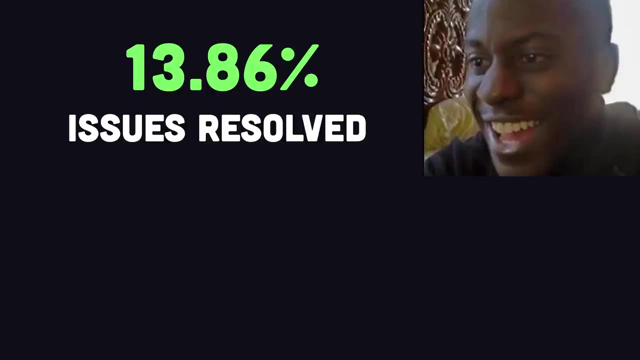 GPT-4 only gets the job done 1.74% of the time, while Devin is currently sitting at 13.86%. That's a huge improvement, but a tool that can only solve GitHub issues 13% of the time is not quite good enough to replace most software engineers today. 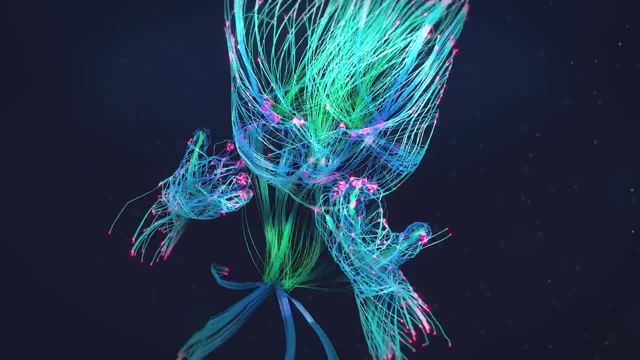 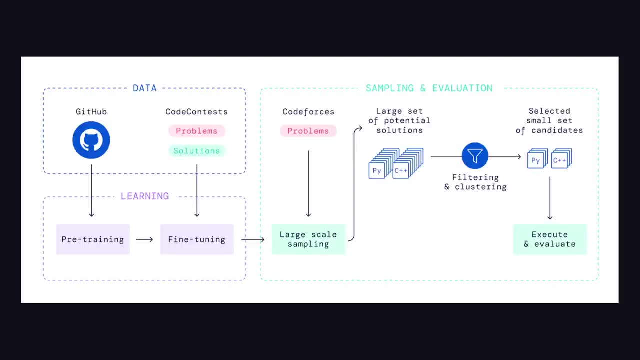 Although this number will likely improve in the future, Things are going to get really long. The only way to handle it, though, when tools like this start doing everything in parallel, like Google's AlphaCoder, which currently beats 85% of competitive programmers, and it does that by using an LLM to generate thousands of possible solutions in parallel. 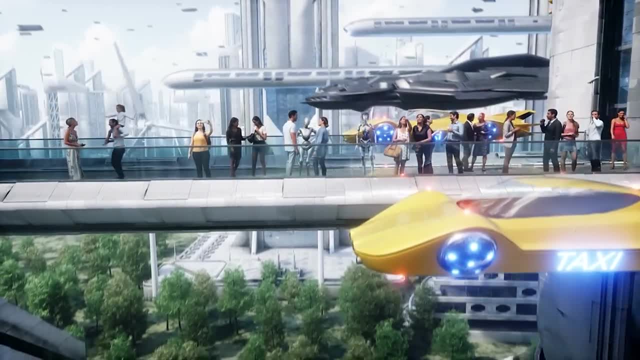 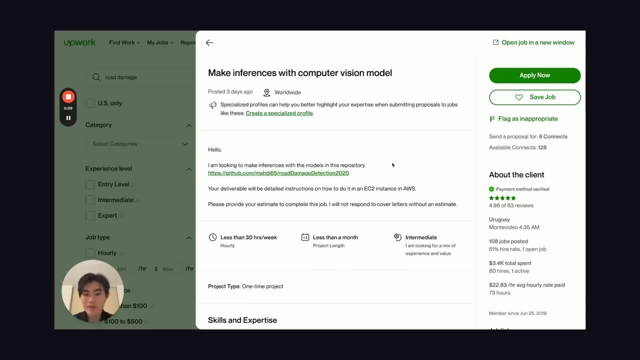 then picks the best one. In the future, you'll be able to post a job just like you would on Upwork, and 10 minutes later Devin will come back with a thousand different apps and you can choose the best one. In fact, Devin is already doing real jobs on Upwork and getting paid for it. 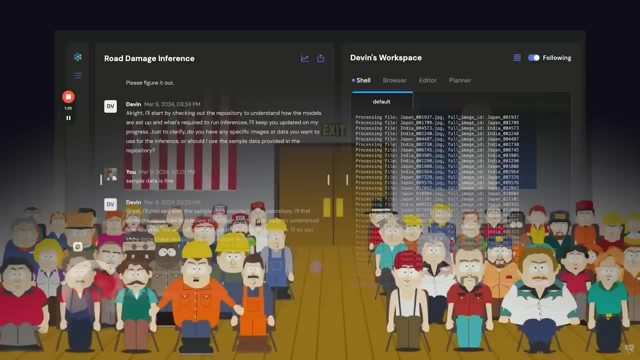 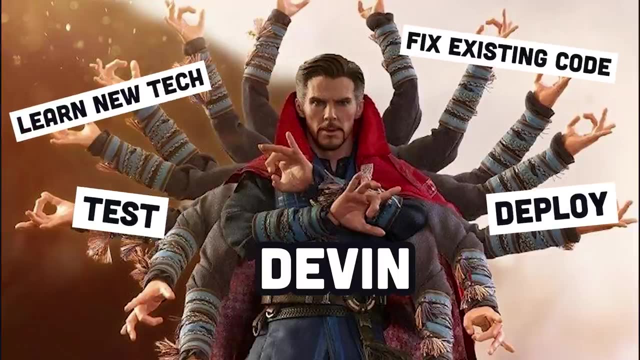 So I guess that makes it official: they took our jobs, They took your jobs. Devin can learn new technologies. it can build and deploy apps. it can fix bugs in existing codebases, train its own AI models, train its own AI models, train its own AI models and do all kinds of other stuff. 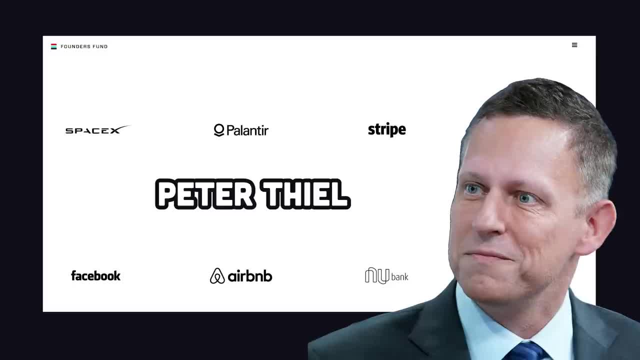 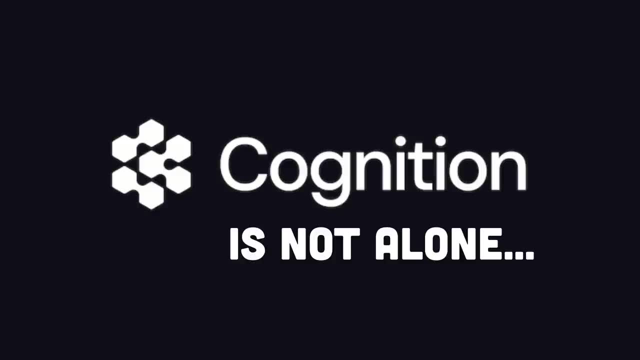 Pretty impressive, and the company itself is backed by Peter Thiel's Founders Fund, along with the Collison brothers from Stripe and a bunch of other heavy hitters from Silicon Valley. And Cognition is not the only stealth startup in this game.